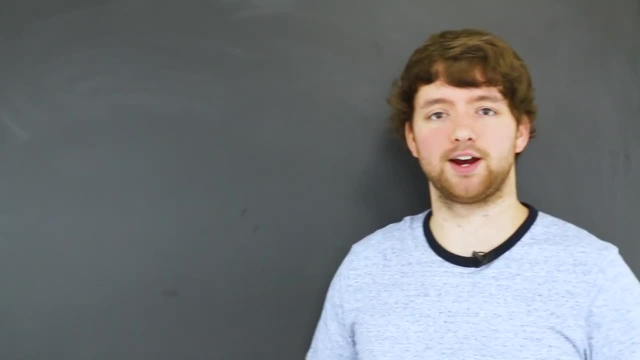 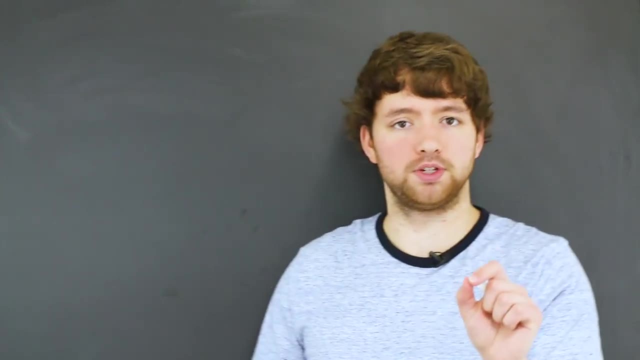 that's going to be great if you need to study or prepare for a job. So be sure to check that out. You can get all the notes in the crash course. Okay, so this video we're going to talk about loops. Now loops: they are dangerous because you can create. 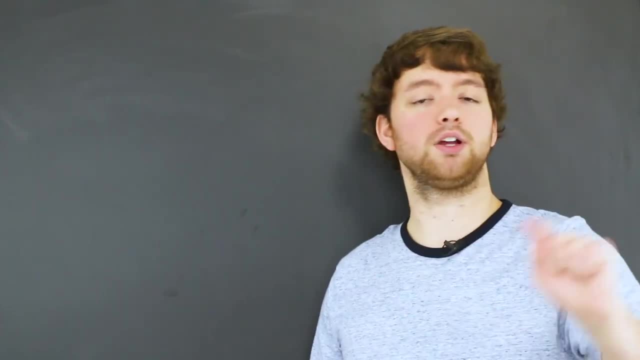 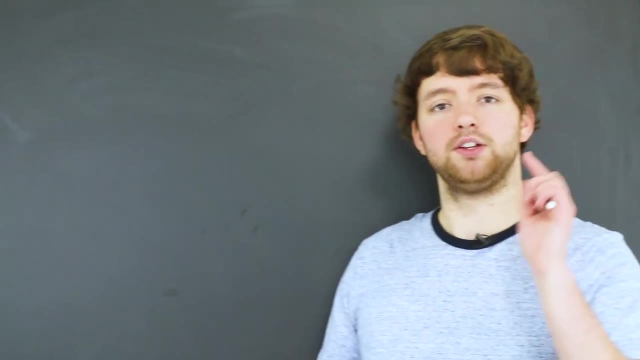 what's known as an infinite loop, where you basically just execute the same line of code over and over and over again until your computer explodes, which is what we don't want to do, right? So we have to be very careful in how we structure our loops. There are three things. you 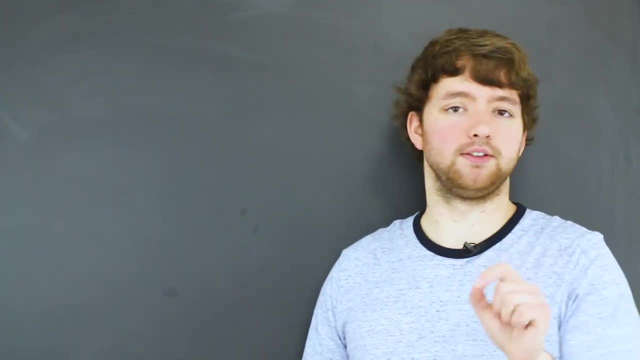 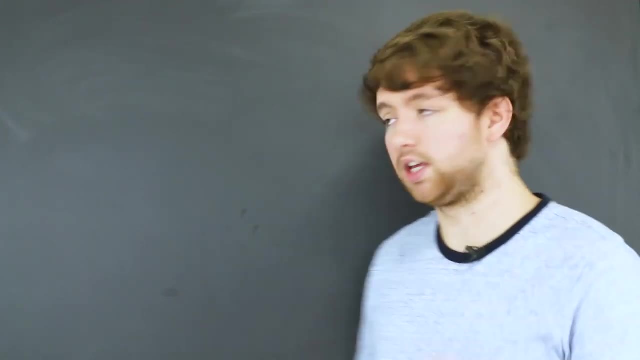 need to consider when making a loop, And then we're going to be talking about the different types of loops And then in the upcoming videos we're going to be doing hands on with these loops. So the first thing is the practice making them. So the very first thing is the initialization. 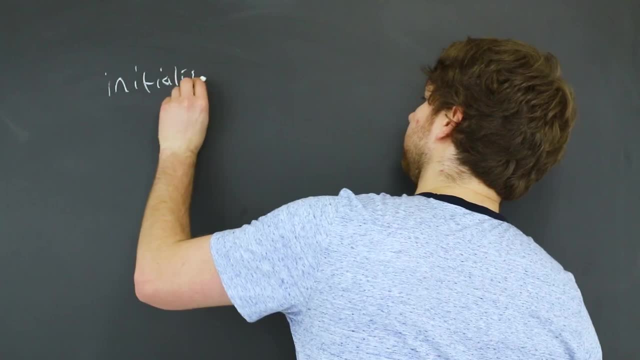 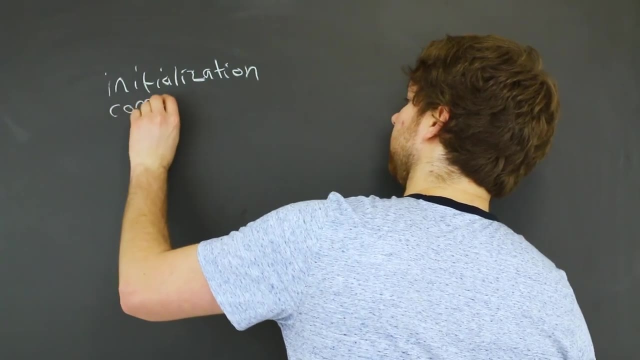 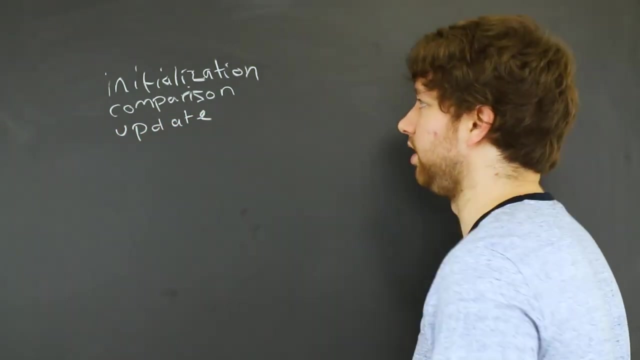 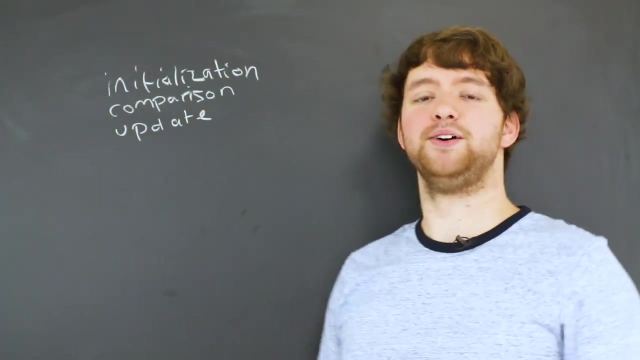 The next thing is the comparison And then the update, And one of my computer science teachers explained that I could remember this. I see you- which I don't know if that's going to help anybody or not, but it works. So what exactly does this mean? So when we want to do a loop, we need to figure out when we're 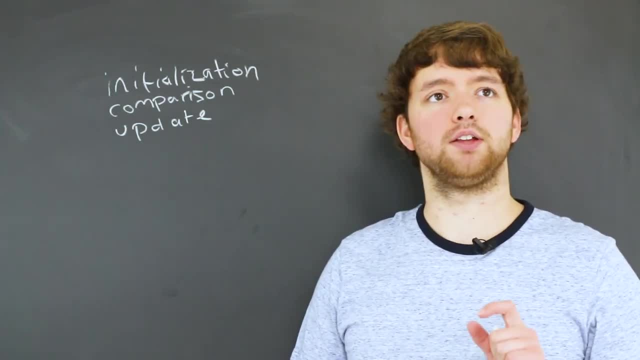 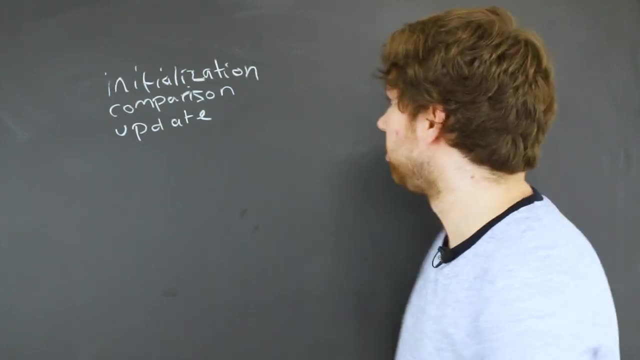 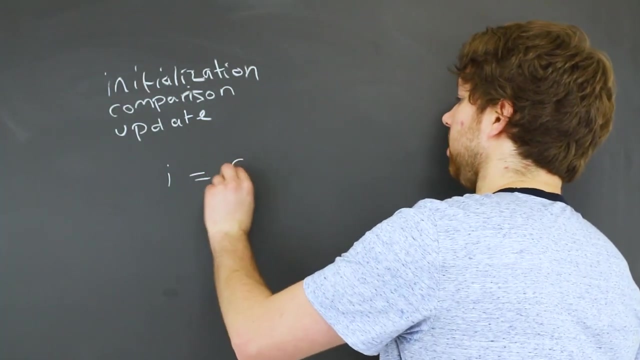 going to start and stop the loop right. So like, let's say, we want to execute something a certain number of times, we need to say when we're going to stop. So the first thing we do is we set the value of some variable to a number. like, let's say, I equals zero. that is initializing, because 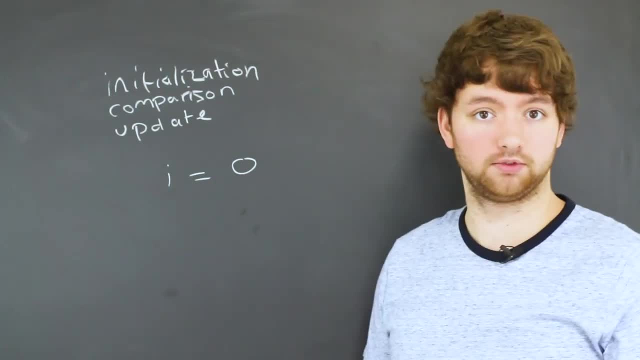 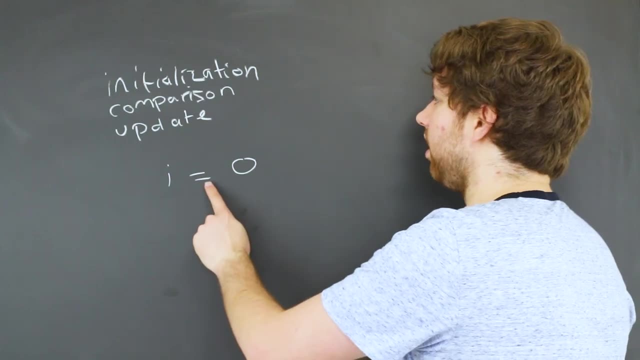 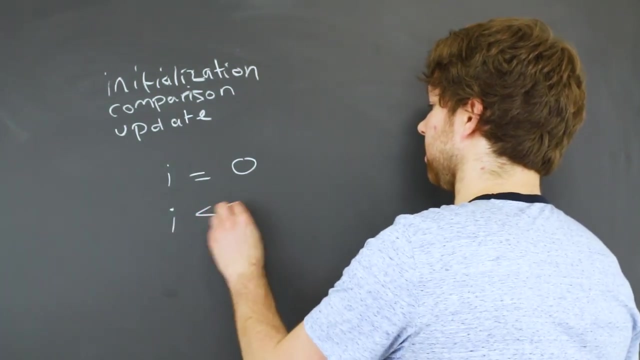 we're saying, hey, I is zero. We initialize the variable And if this doesn't make any sense, just wait it will. I is zero. And then we want to increase I until we get to I is less than or equal to 10,, for example. So this is: 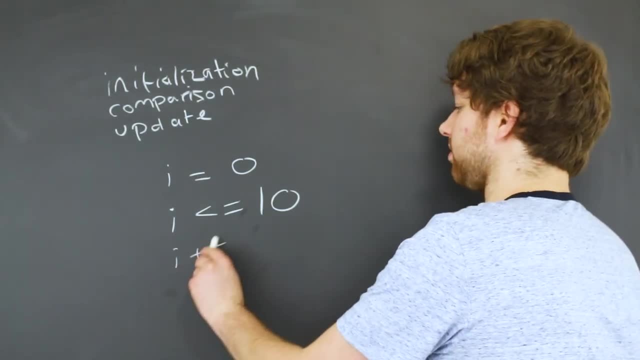 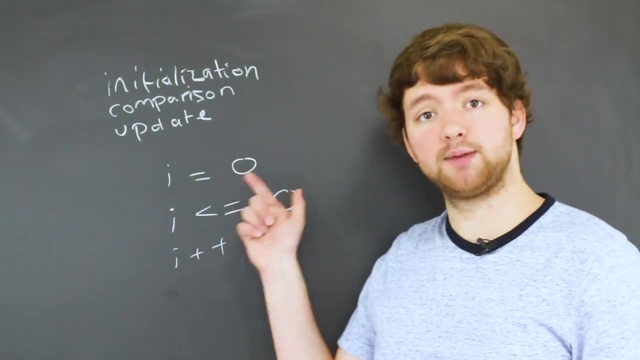 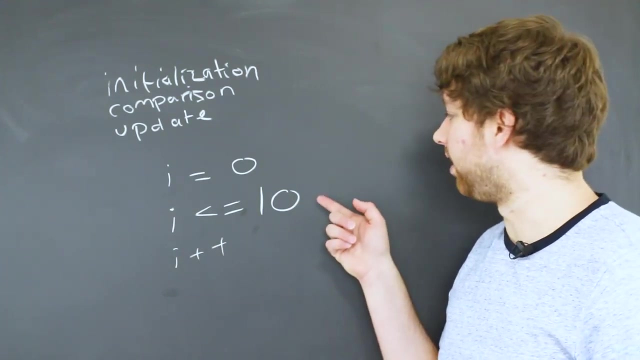 the comparison And then the update is I plus plus. So here are all of the pieces. we start at zero. we're going to keep doing the same thing Until I is less than or equal, or while I is less than or equal to 10. And then every time we do it. 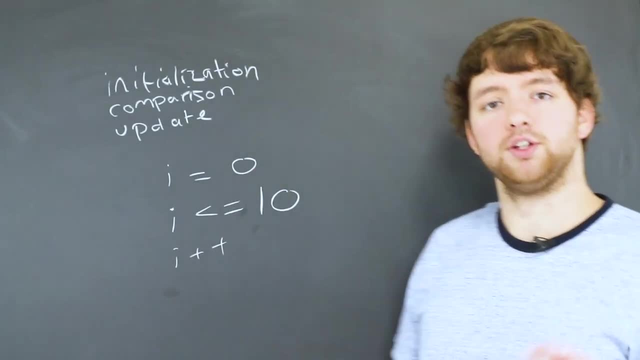 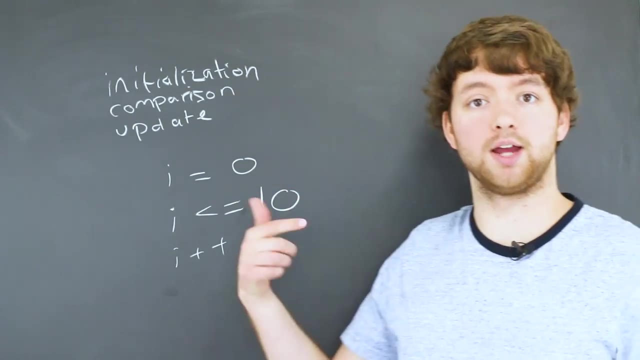 we're going to increase I one time So you can see how this makes a loop. we say where we're starting, how we know if we're continuing and what we're going to do after each time so we get closer to finishing. So these are the three pieces And it can be a little bit confusing at first. 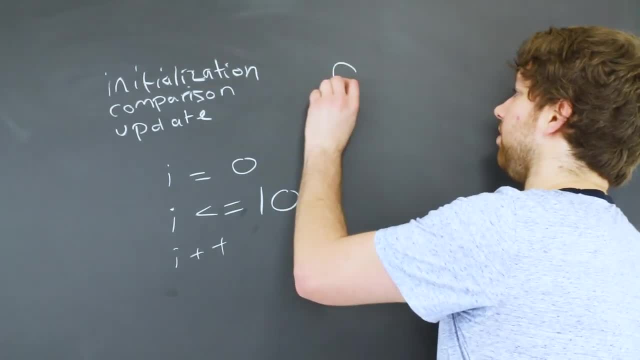 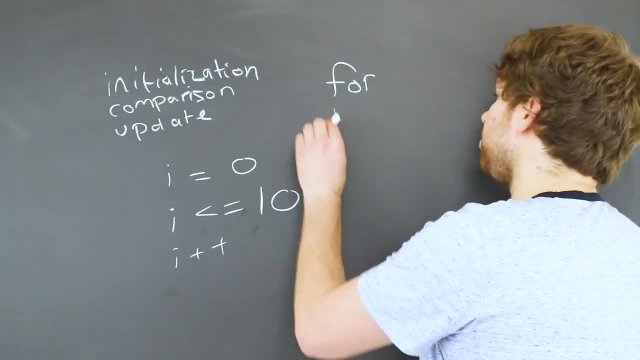 But once we go into the next videos, we're going to be talking about the for loop. you're going to be able to do that, And then we're going to do that, And then we're going to do that, And then we're going to visualize all this very simply and create a simple loop. There are also two other. 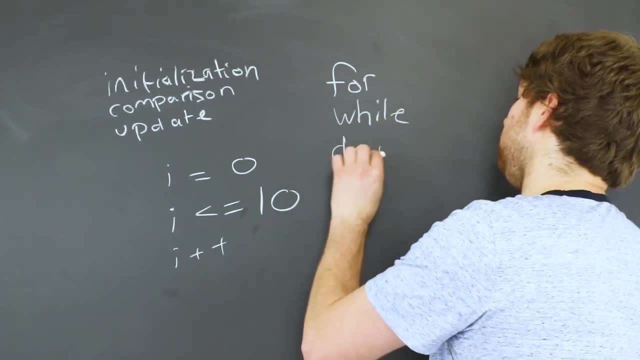 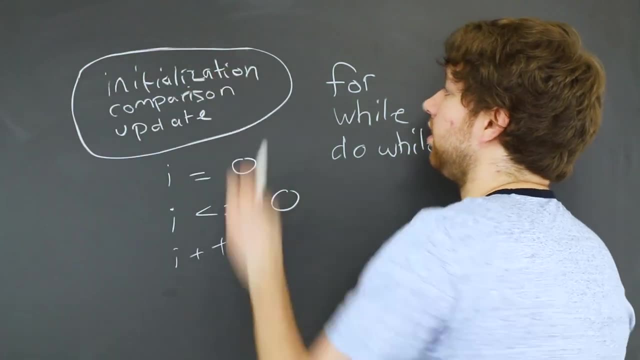 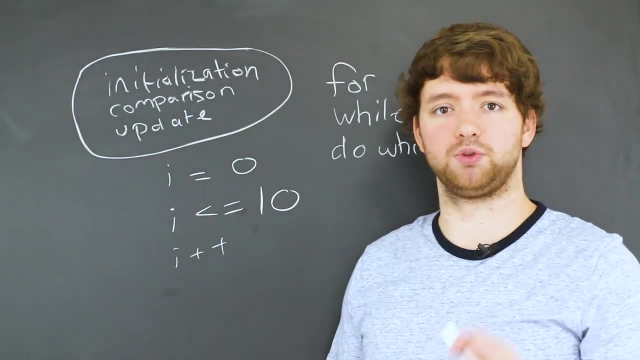 loops, which is the while loop, and do while loop, which what all of these have in common is they all need these three things to not create an infinite loop. So guys go check out the upcoming videos, because we're going to be breaking down loops and making them very simple. So far, we've talked. 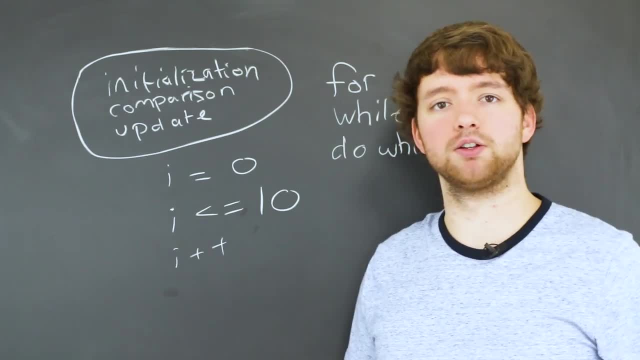 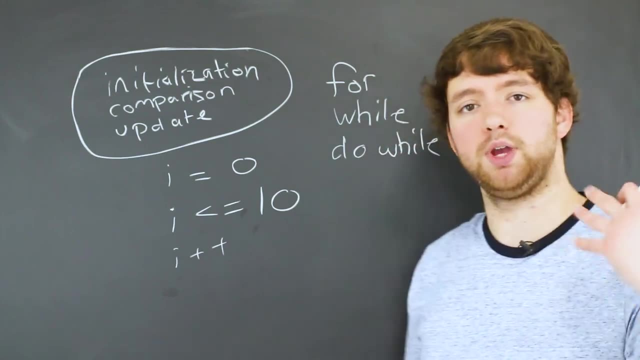 about if statements switch statements and turn on and off, And then we're going to talk about these as Oooh and two other loops, a loop that's called books, a paper loop, And take note, there'sço are down a little more than three unabsorbed elements here and we are talking about 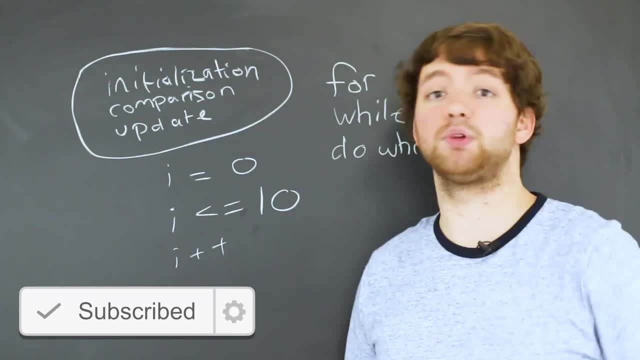 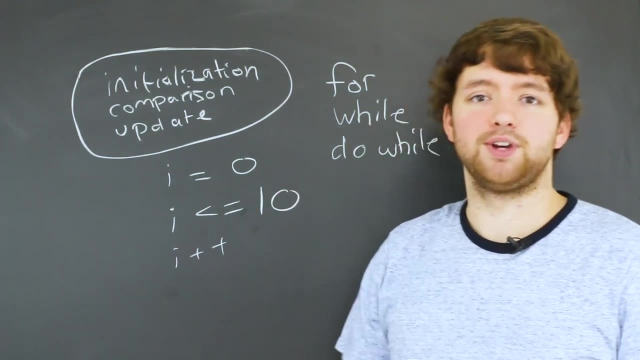 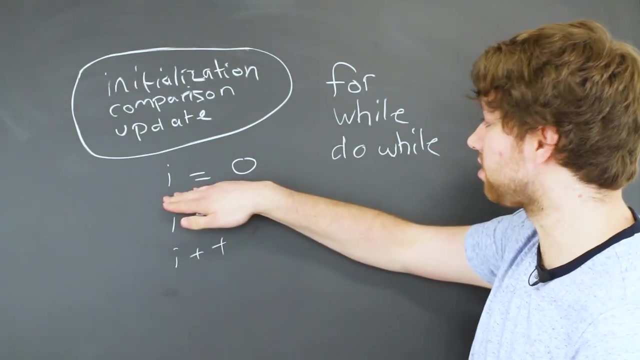 this loop around loops and levels. So this loop marks how we're going to make a loop or a loop out of it, right? So we're going to walk over to something that is my dozens and I'm going to talk about how to make one of these structures gives us very simple examples of when we need. 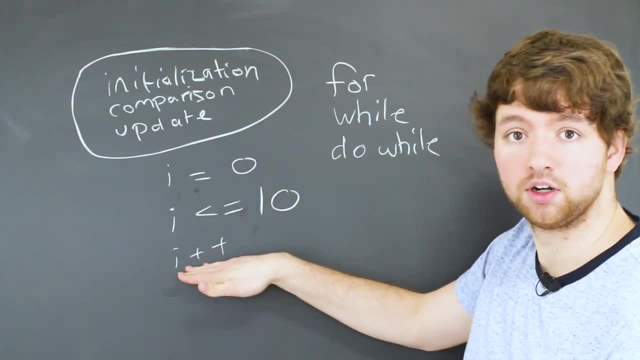 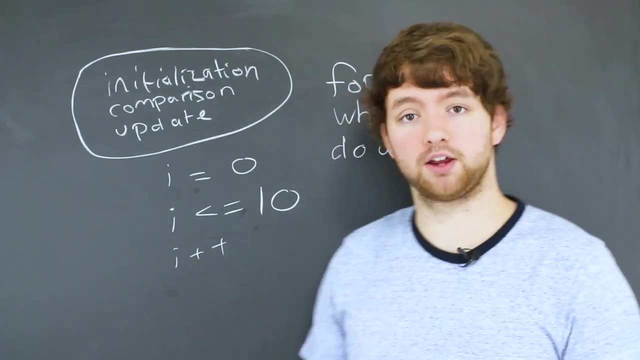 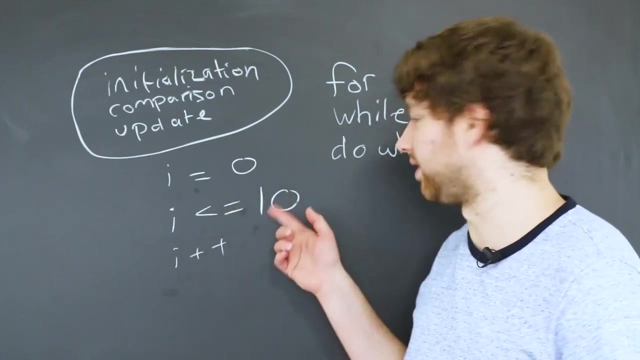 these and then we increase some number until this condition is no longer true. You can think of it like going around a race car track: We start with zero laps. Every time we go around, we increase our number of laps and we stop when we get 10 laps. So as long as it's less than 10,. 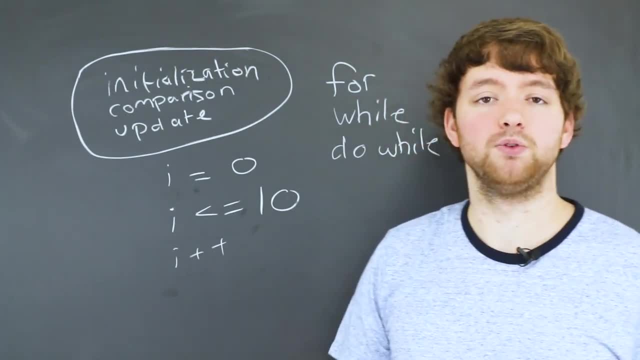 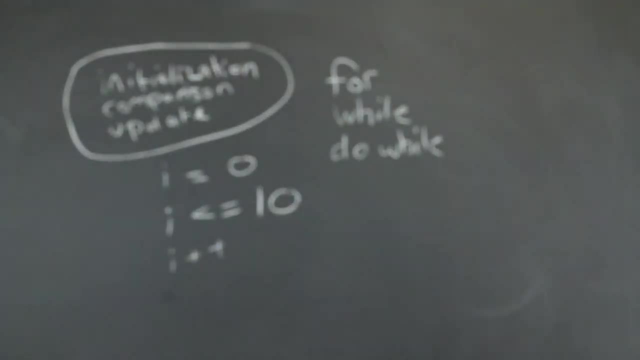 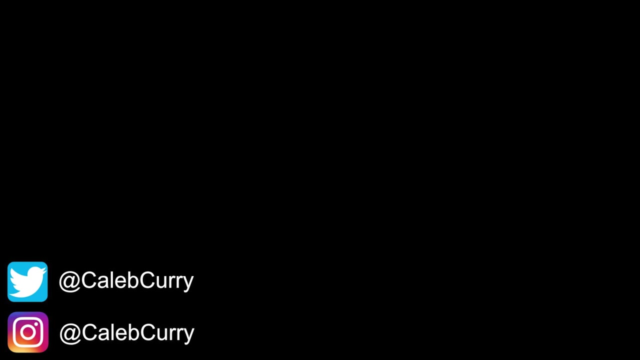 we keep driving. So thank you guys. Hopefully that was helpful. Please be sure to subscribe. Definitely helps me out and I appreciate every time someone subscribes. So thank you and I'll see you in the next video. Thanks for watching.